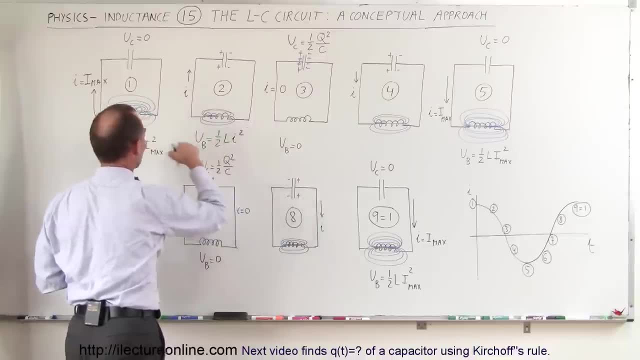 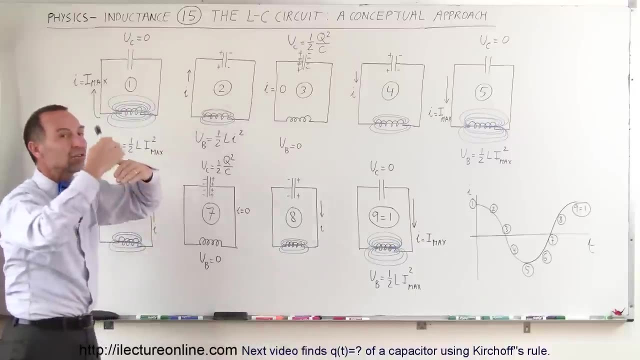 is now going to be one-half Li squared, where I is, of course, less than the maximum I, So the energy on the inductor begins to diminish and the energy on the capacitor begins to increase. The amount of energy on the capacitor at that point will be equal to one-half. 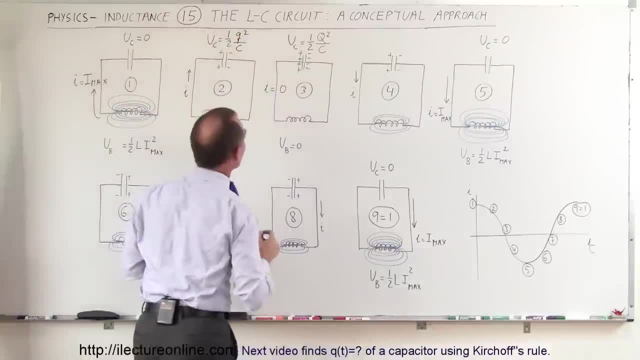 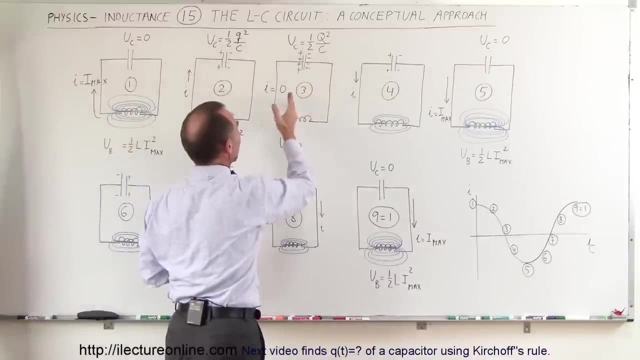 times the charge on the capacitor squared divided by the capacitance. Eventually the capacitor will get fully charged. maximum charge will build up on the capacitor. At that point the current will stop. It's basically the current will stop. the capacitor now fully charged. 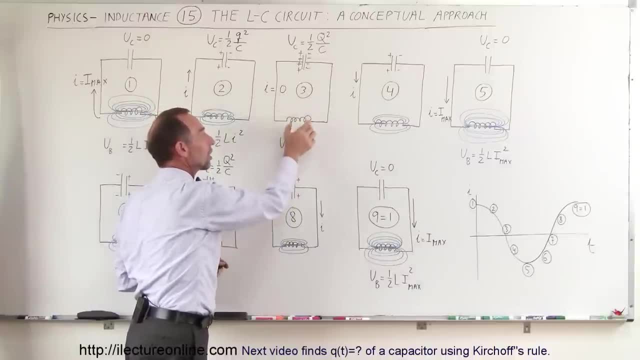 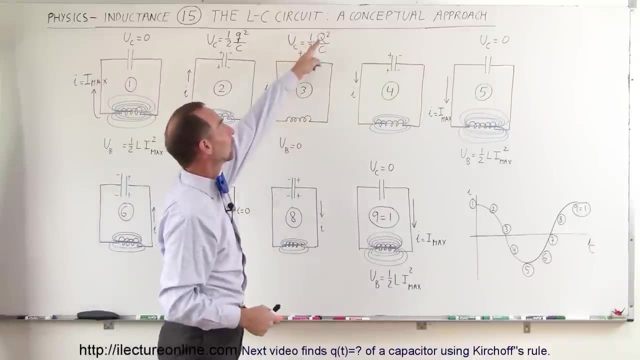 Since there's no current flowing in the circuit, there's no magnetic field in the inductor, so the energy in the inductor is zero and the energy in the capacitor now has reached its maximum value. It's equal to one-half times the total charge on the capacitor squared, divided by the capacitance. 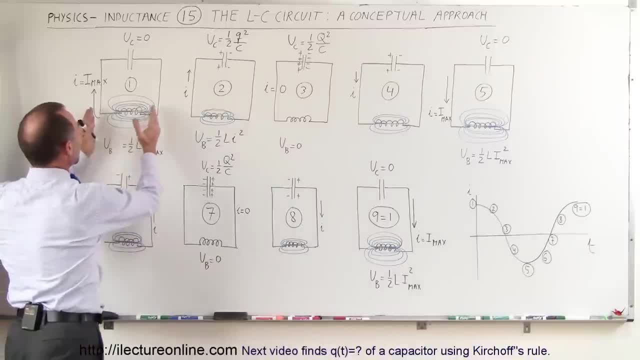 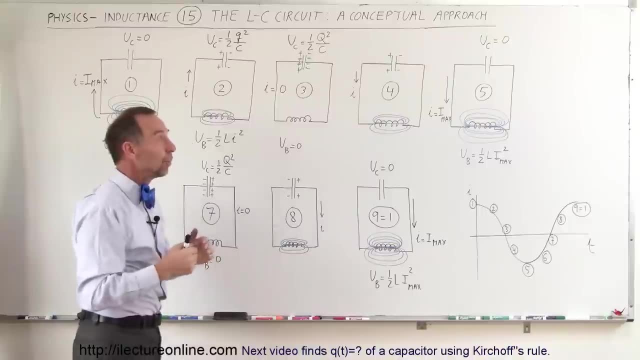 The energy that was stored on the inductor, the exact same amount will now be stored on the capacitor. So all of the energy is transferred from the inductor to the capacitor. At that point the capacitor begins to discharge. Current is beginning to flow back in this direction. 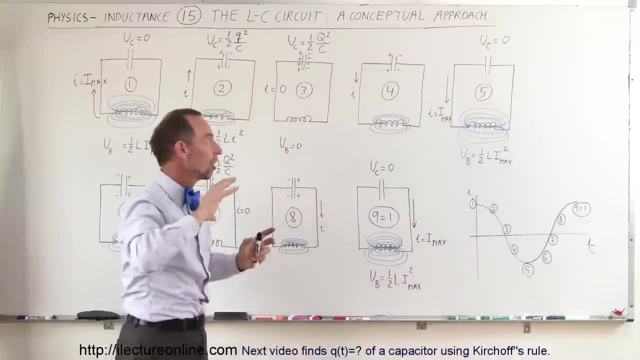 Remember, there's energy stored in the capacitor. It pushes that charge back into the circuit, back through the inductor. The inductor tries to oppose the change in current. By doing so, it starts building up a magnetic field, It starts building up energy. 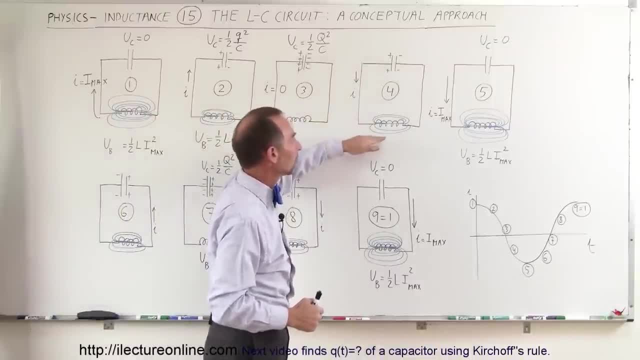 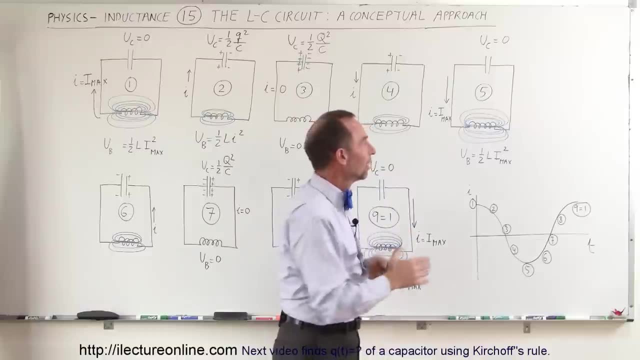 Energy begins to dissipate out of the capacitor as charge is being pushed back into the circuit And eventually the maximum current will be reached. when the capacitor is now fully discharged And the maximum current is reached, therefore, we now have maximum energy in the inductor. 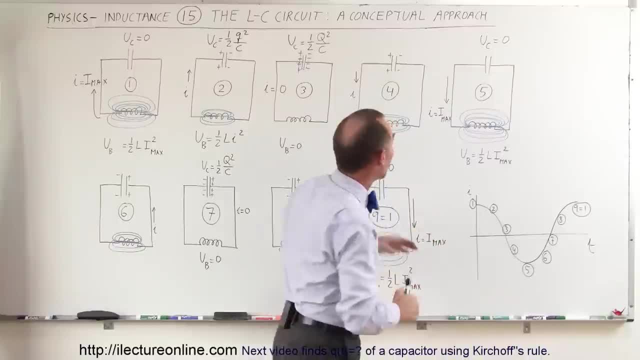 The capacitor has zero energy. the inductor now has maximum energy. All the energy that was in the capacitor here has now transferred into energy in the inductor. But since the current was slowing at its maximum, it's not going to stop instantaneously. 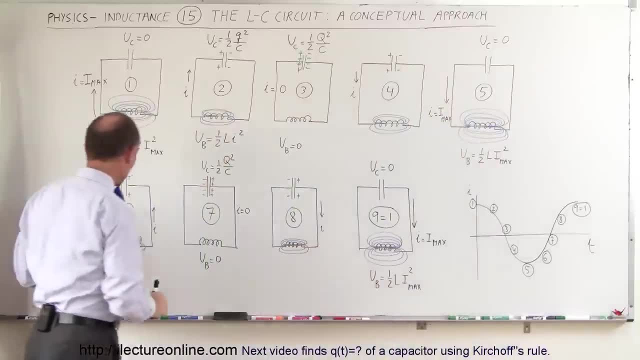 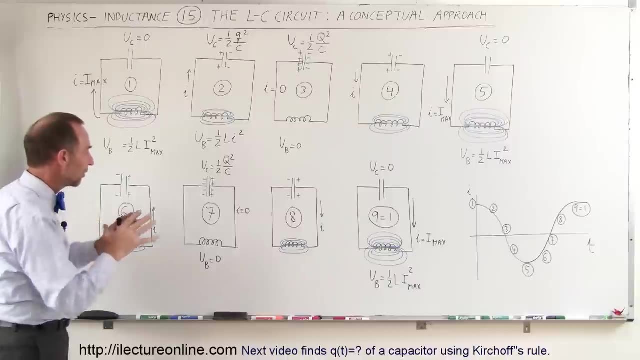 it's going to keep on flowing, as we can see here, which now means that charge is now going to pile up on the other side of the capacitor. As its charge begins to fill up, it begins to push back against the current. The current begins to diminish, but the inductor is going to continue pushing the current through the circuit. 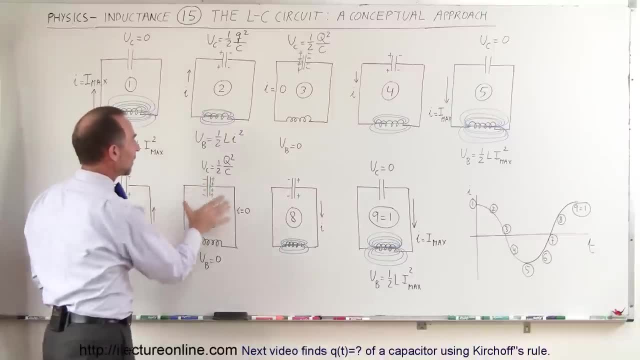 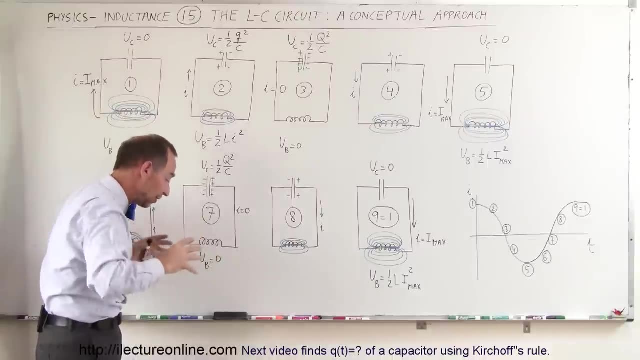 until the capacitor is fully charged. At that point we have maximum energy in the capacitor- again one-half Q squared divided by C. zero energy in the inductor because all the magnetic field is being used. and we have zero energy in the inductor because all the magnetic field is being used. 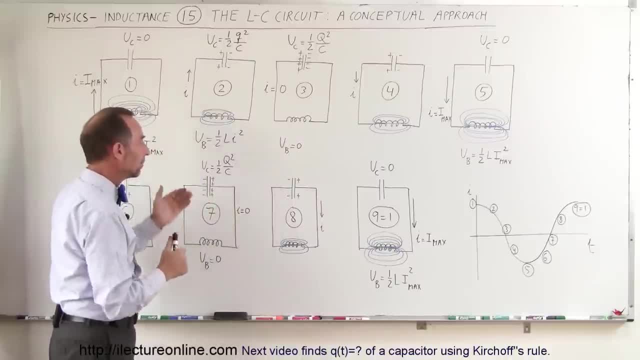 and we have zero energy in the inductor because all the magnetic field is being used to push all the current back onto the capacitor. At that point the capacitor begins to push charge back in the opposite direction. The magnetic field is going to build back up in the inductor. 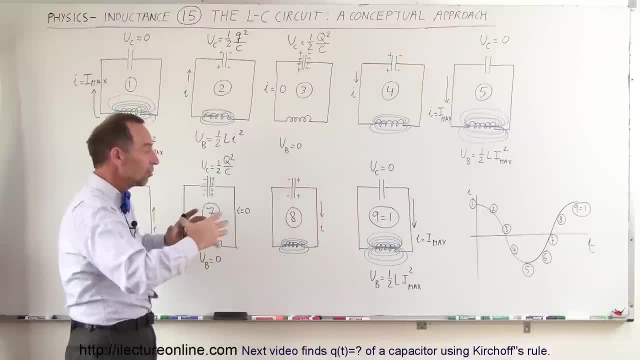 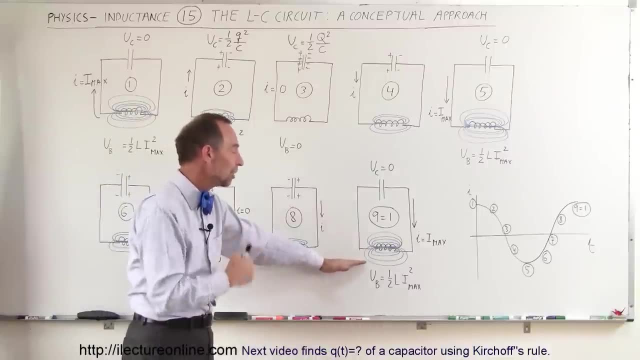 as it's beginning to oppose that change in the current. It begins to increase its content of energy as the magnetic field builds up, until it fills up to its maximum energy capacity. That's when the maximum current is reached. That's at the point when there's zero charge on the capacitor. 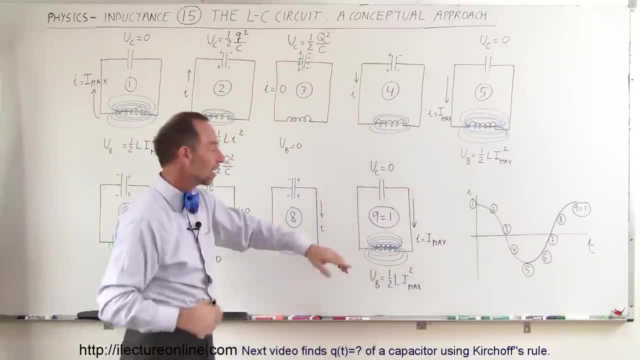 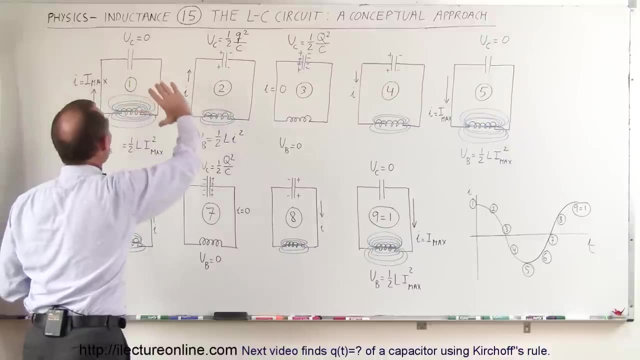 We now have maximum current in the opposite direction, We have maximum magnetic field in the inductor, therefore maximum energy. At that point we're back to the point right here where the current will continue to flow through to the capacitor. It begins to charge up and the whole process starts over again. 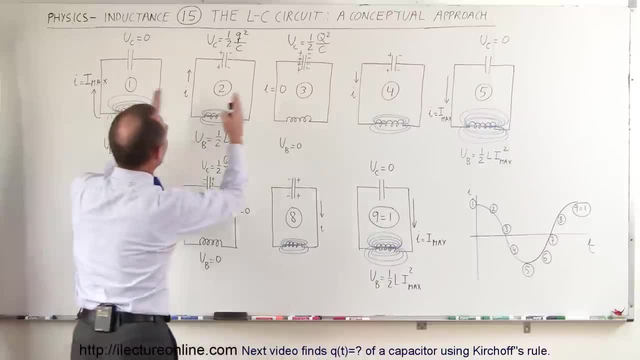 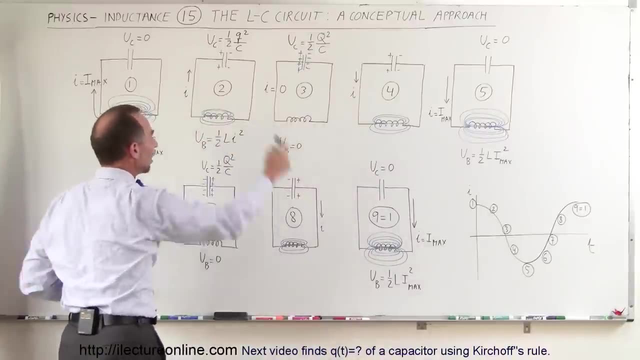 What will happen is that charge will flow into the capacitor. The capacitor will push all the charge of the inductor back to the other side and back to the first side and back to the other side. The current will go back and forth and back and forth and back. 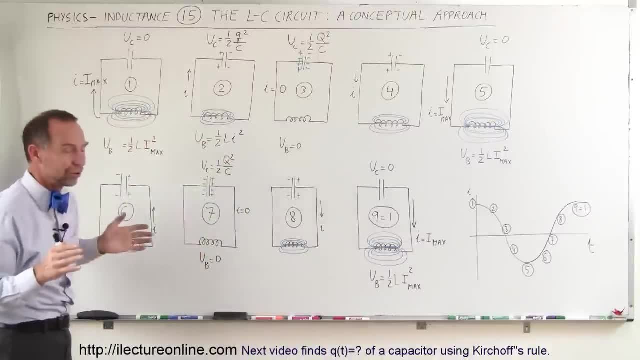 The current from the capacitor drives the charge in the inductor back and forth and forward. Assuming that there's no resistance in the circuit- which of course in the real world that doesn't exist- there's always going to be some small amount of resistance, even if all you have are conductors. 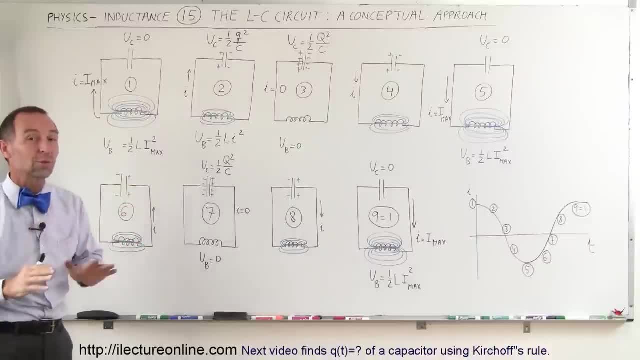 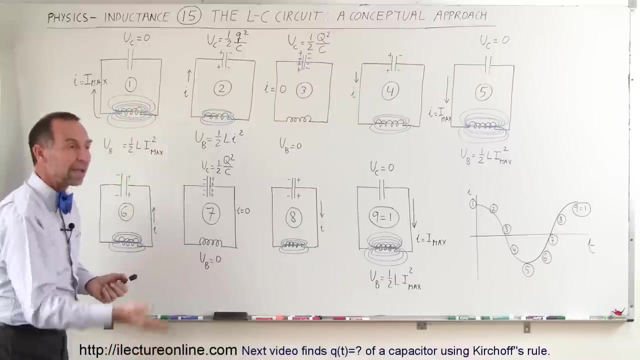 But if you assume for a moment that it's a perfect conductor, there's no resistance whatsoever in the circuit. this oscillation back and forth would go on forever and ever, and ever. And it's very analogous to a mass on a spring. You put in potential energy by extending the spring you let go. the mass is now going to flow back and forth. 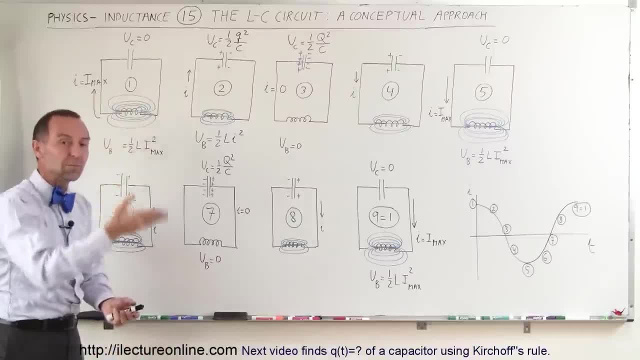 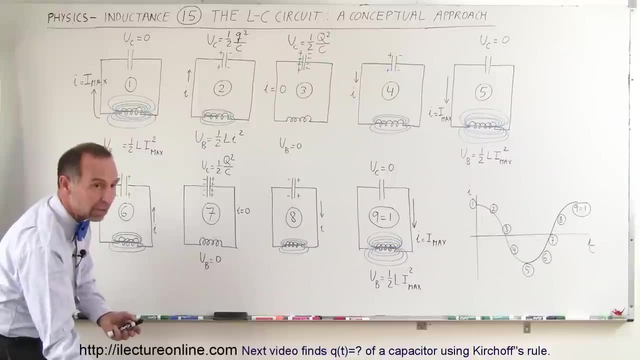 and the energy exchange is going to be between potential and kinetic energy. potential and kinetic energy as it goes through its equilibrium point, to the opposite side, back to equilibrium point, back to maximum elongation, back to equilibrium point, back to maximum compression, and so forth. 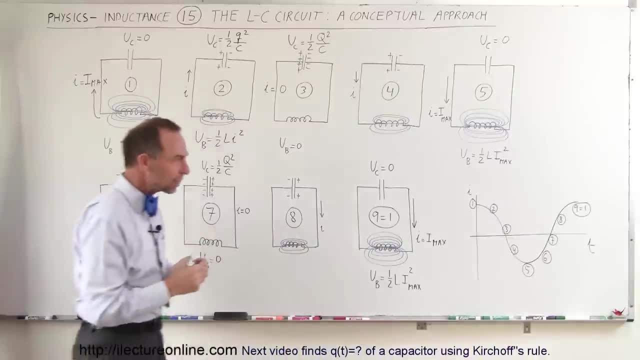 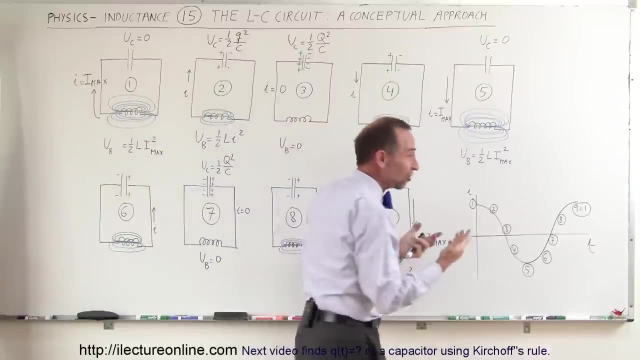 It is exactly analogous to that. If we take a look at what the current flow looks like in case number one, we have maximum current in the clockwise direction. let's just call that a positive direction, doesn't matter. Then of course, the current is going to be diminished.